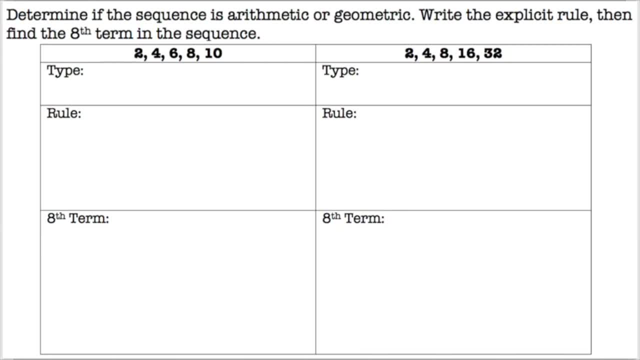 geometric. Write the explicit rule, Find the eighth term in the sequence. So on the left-hand side we have two, four, six, eight, ten. So we can first check to see if they're adding a certain amount And then if they're not. 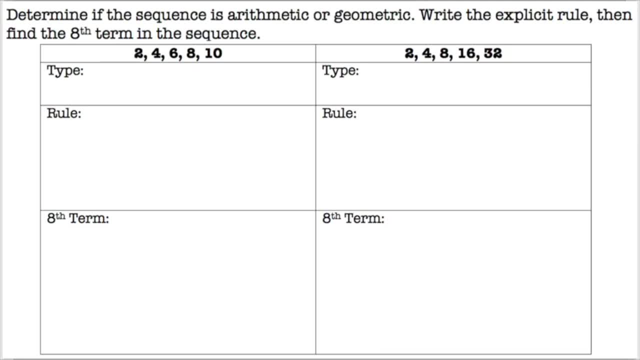 then we check to see if they're multiplying by a certain amount. So two to four is a difference of two, Four to six is a difference of two, Six to eight is a difference of two, And eight to ten is a difference of two. So that means it is arithmetic, because you're adding And then the rule is that 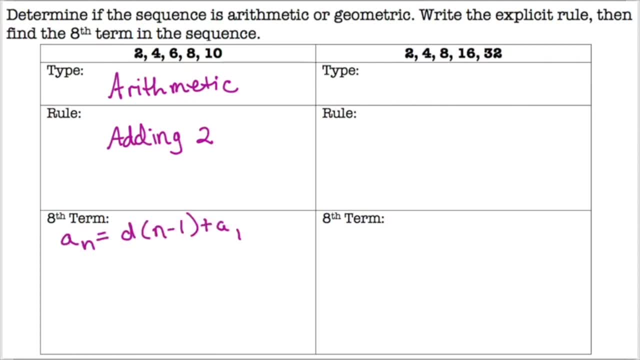 adding two. So then if we're finding the eighth term, we're going to use the arithmetic sequence formula, which is: a sub n equals d times parentheses, n minus one plus a sub one. So we just plug in things that we know. So our d is going to be the adding two And then n is going to be what the 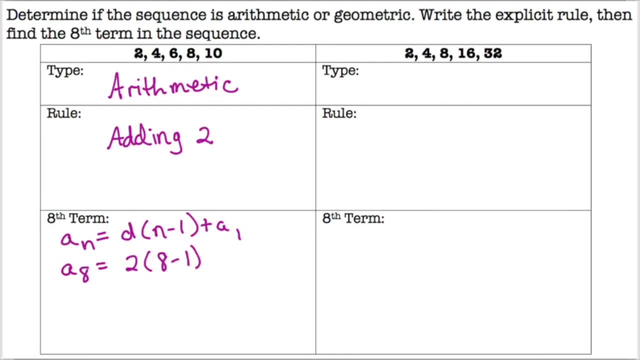 sequence we're looking for, which is eight, And then a sub one is the first number in the sequence, which is two. So you do two times eight and two times negative One first. So that's 16 minus two. Bring down the plus two and then just add and subtract, So 16. 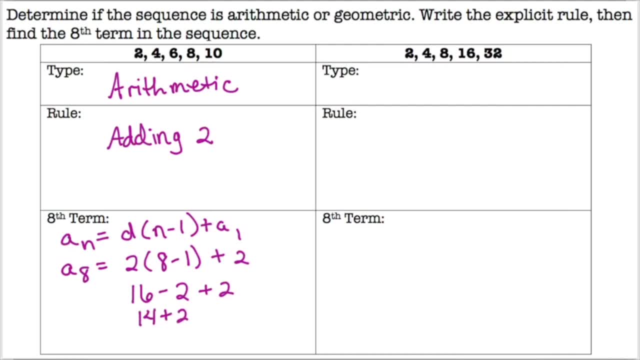 minus two is 14.. 14 plus two is 16.. So then a sub eight is equal to 16.. On the right hand side, two to four, four to eight, 16 and 32.. That is geometric, because it's multiplying by two each. 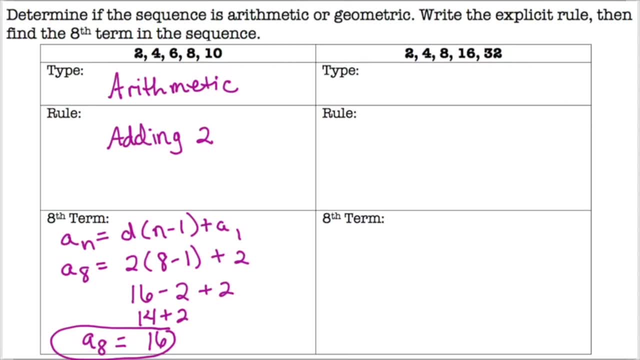 time, And you can find that by Trying to see if there is a common difference by subtracting. So four minus two is two, but eight minus four is four. So that doesn't work. So then you have to do four divided by two. 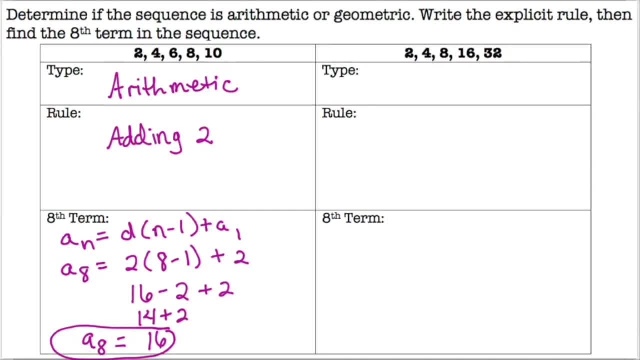 which is two, and eight divided by four, which is also two. So we know it's geometric. So then, for that, you're going to multiply by two, And then, the eighth term, we're going to use the geometric sequence formula, which is a sub, n equals a sub one times r raised to the nth. 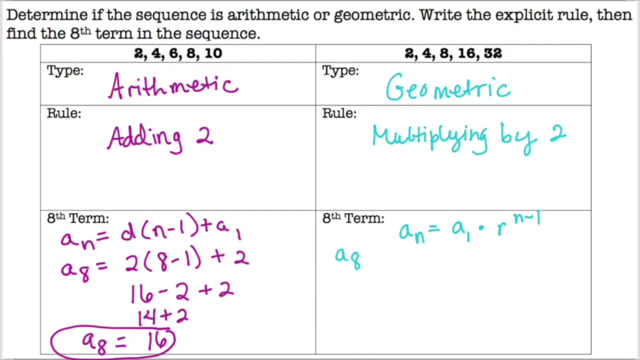 Minus one power. So we're going to find a sub one which is two. That's the first number in the sequence times. the ratio which we just found was also two, And we're looking for the eighth term. So we're going to do eight minus one, which two raised to a minus one is two to the seventh. 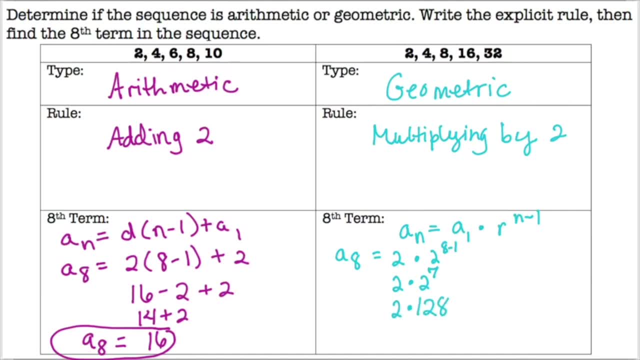 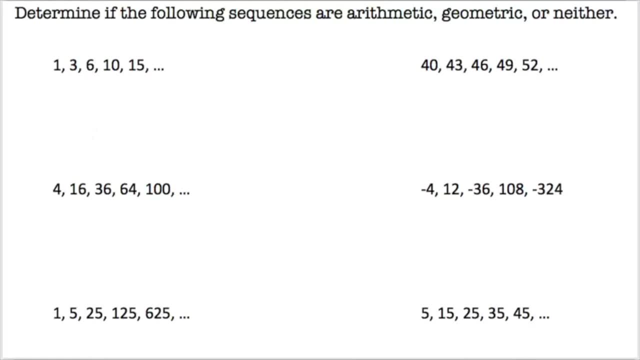 power to the seventh power is 128 times that by the two in the front And you get 256 for your answer for this side, All right. So for this one we have to determine if the following sequences are arithmetic, geometric or neither. So the first problem: you have a difference between one and three of plus two. 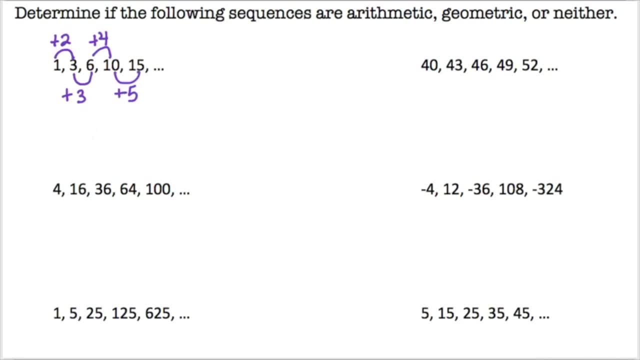 then plus three, then plus four and plus five. So I did it up and down like that, just because the numbers are close to each other and it's kind of hard to write plus next to each other because you get confused. So you don't have to do it like that, You could do it all. 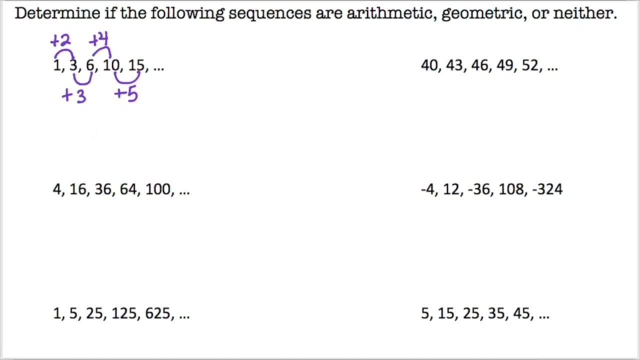 underneath the sequence Um and so the. because they're all different, we have to see if they're geometric. So we know that they're not arithmetic, So geometric we do the division. So three divided by one is three, And then six divided by three is 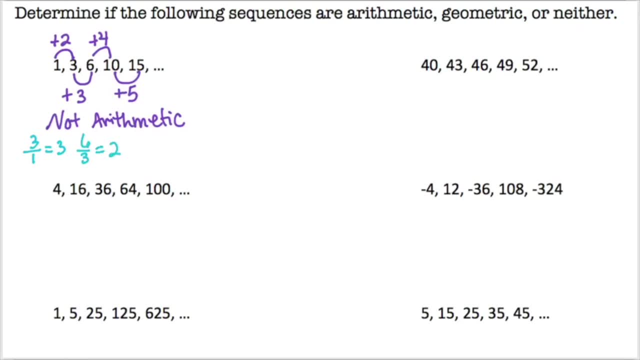 two. We just take the second number divided by the first number, and then take the third number and divide it by the second number. So just right to left. And because those two don't match either, then it's not geometric, So it has to be neither. And then the next one we have a difference of. 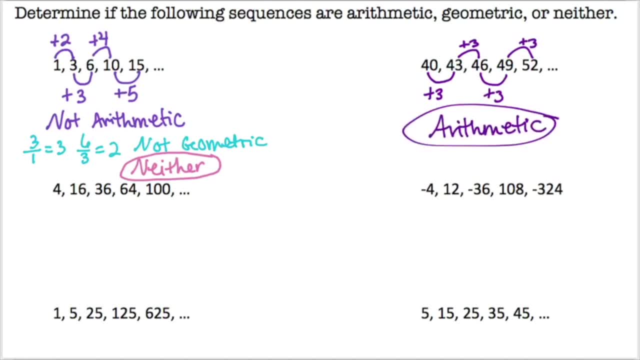 plus three each time. So if it's adding the same amount every time, it's arithmetic. And then for the third one we have four: 16, 36, 64, 100.. So let's check to see if it adds by the same amount, and it does not. 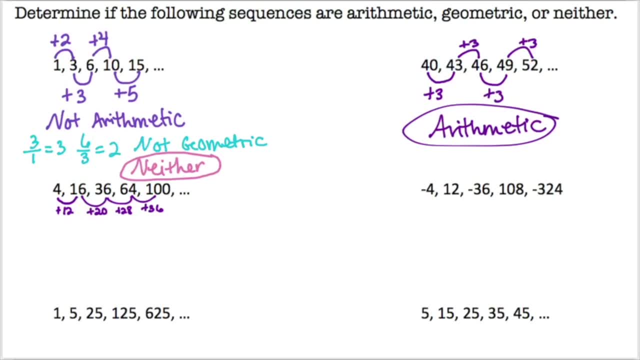 The difference is 12, then 20,, then 28,, then 36.. Then we're going to divide. So 16 divided by four is four, And then 36 divided by 16 is two and a half or 2.25.. Sorry, And those two do not match. 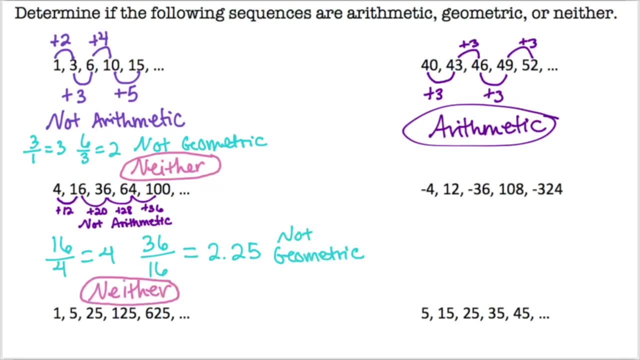 So it is not geometric. So that means it's neither again. And then for number four, we would try to find the difference between adding each time, But for this one actually let me go back one. So for this one we don't even have to worry about the adding one, because look at the numbers, They go negative.